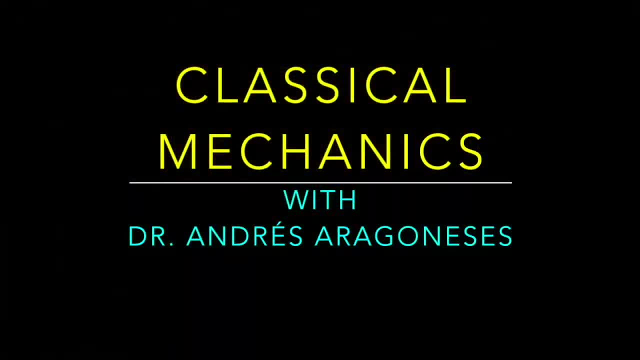 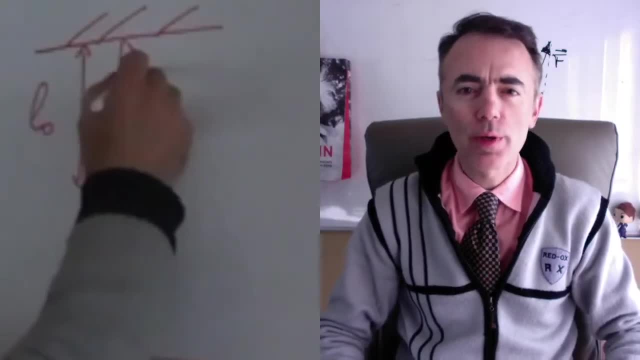 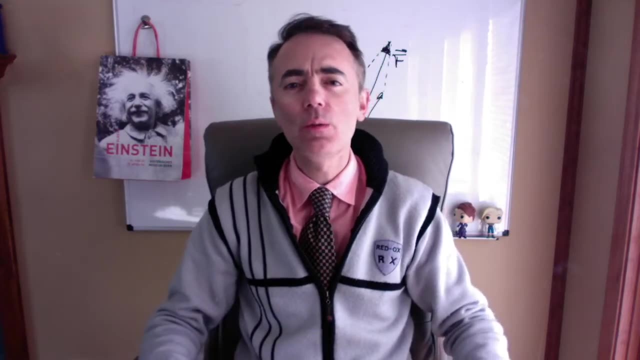 Hi, how you doing. In the previous video I solved the simple problem of two springs and a bob with nonlinear oscillations. Today I'm going to take the same problem, but I'm going to assume that the springs, when they are vertical, they are already. 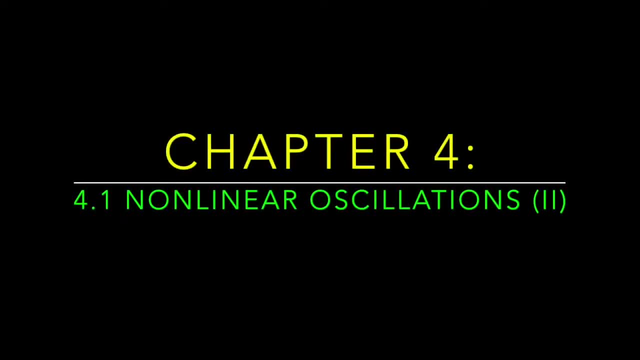 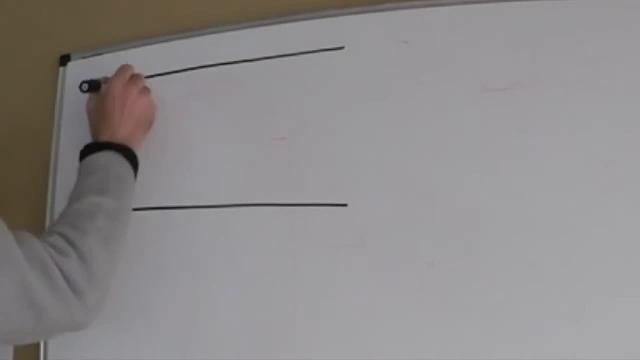 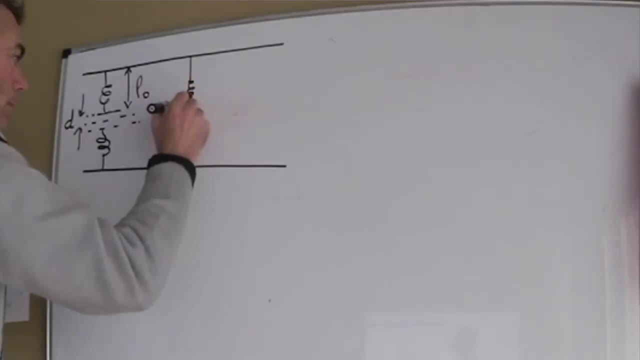 stretched. Consider two springs of elastic constant k on the y-axis. There's no gravity in this problem. We're doing the experiment in deep space. We stretch the springs to join them to a mass m. We then move slightly the mass along the x-. 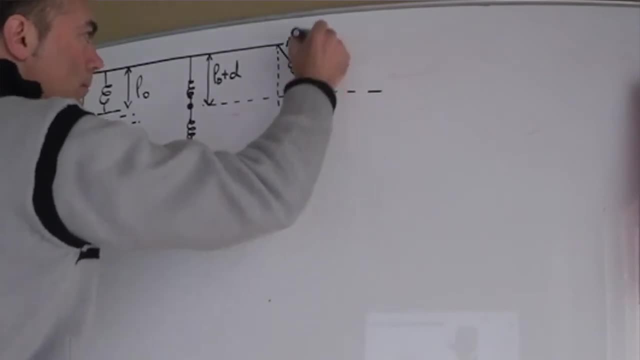 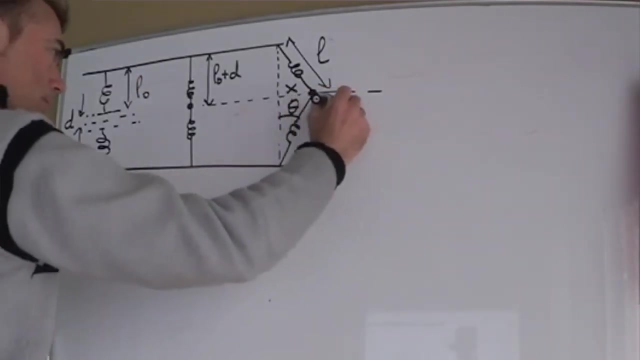 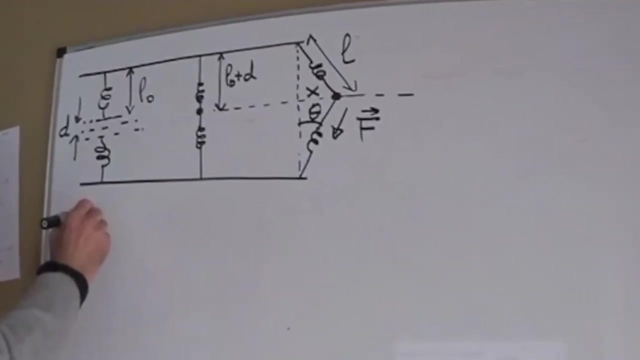 axis and let go, It will start to oscillate. Let's find the effective force on the mass and the related force. First let me write some geometrical relations that might be of use later. L0 is the equilibrium length of the spring without the mass. D is the 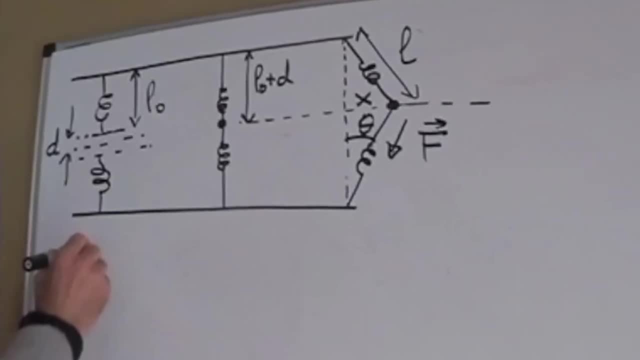 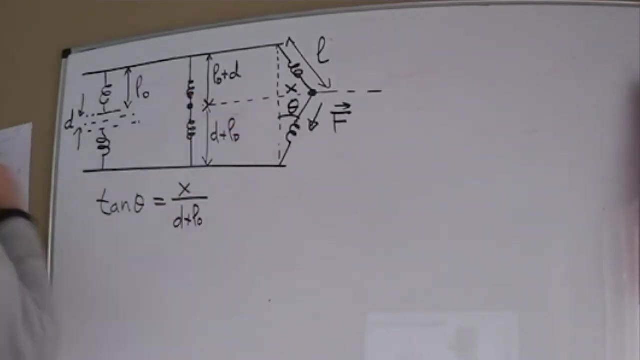 distance that each spring is stretched initially. L is the length of each spring is stretched when the mass is at position x. I define this angle theta, where the tangent of theta is x over d plus L0.. I can also relate L with x, d and. 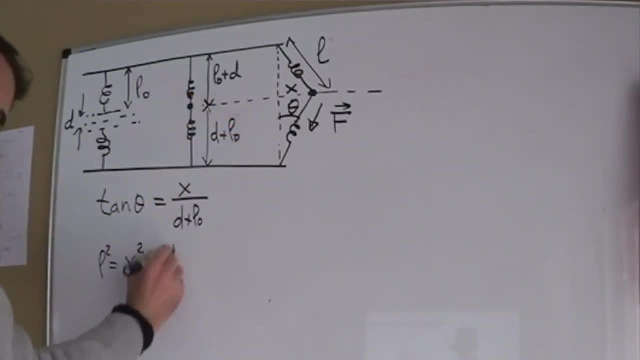 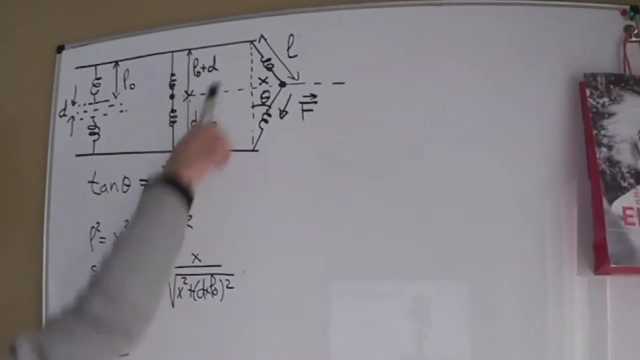 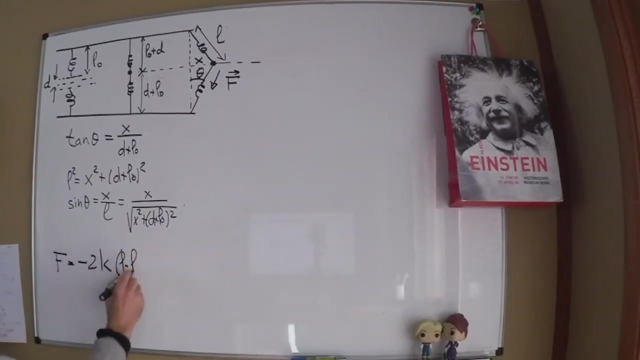 L0 through L square is equal to x square plus d plus L0 squared. Here, sine of theta is x over L, so x over the square root of x squared plus d plus L0 squared. Now let's write the force on the x-axis: f sub x. F sub x is equal to minus for the recovery. 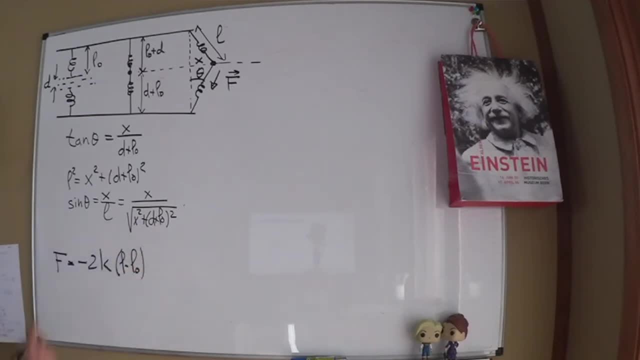 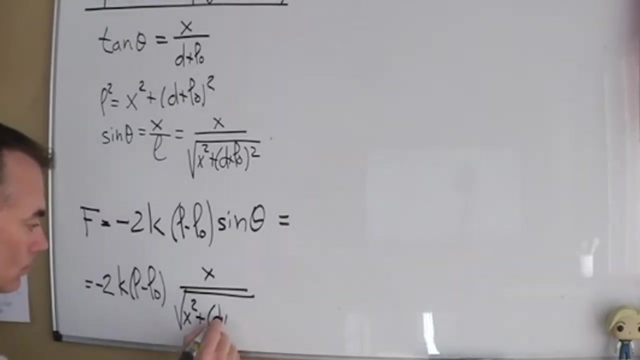 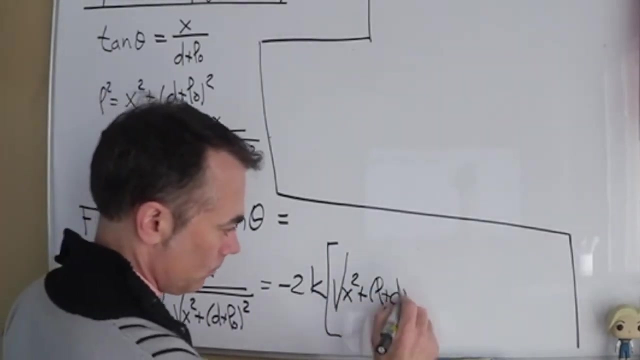 force two, as there are two springs, K, L minus L0, which is the amount of force that is stretched of the spring times, the sine of theta For the projection on the x-axis. I substitute the sine of theta here. I also substitute the length L here. 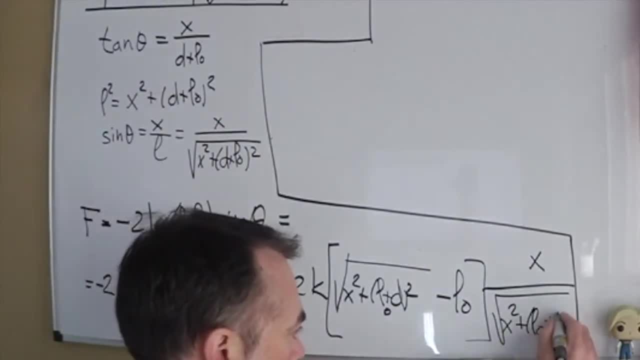 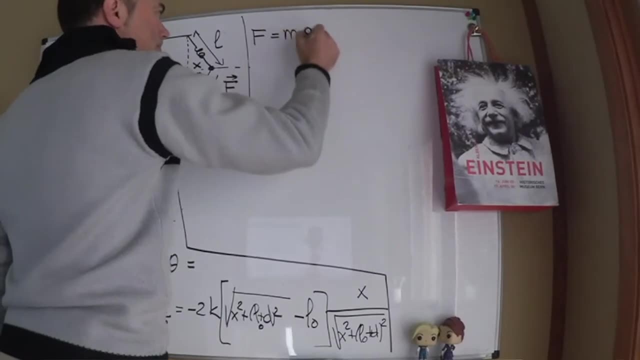 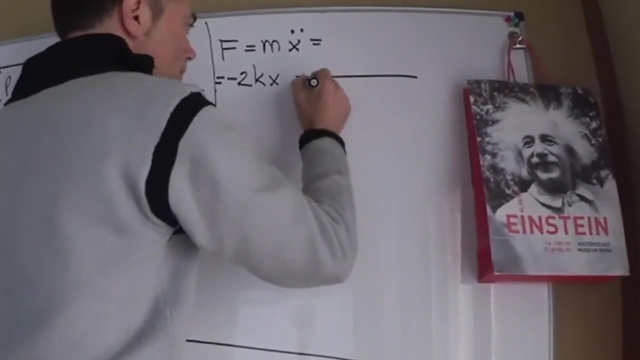 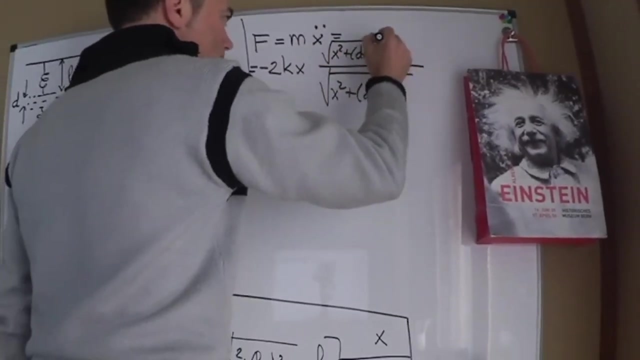 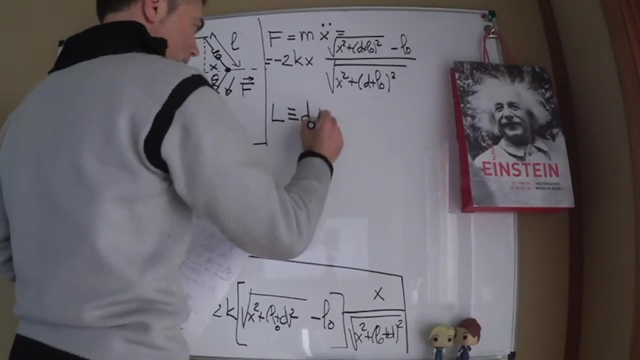 So the force f sub x is this questionably beautiful expression. So we have the mass which is oscillating along the x-axis, which follows Newton's second law. f sub x is m times x, two dots. Now let me call d plus L0 as capital L, so I can simplify a bit the looking of this. 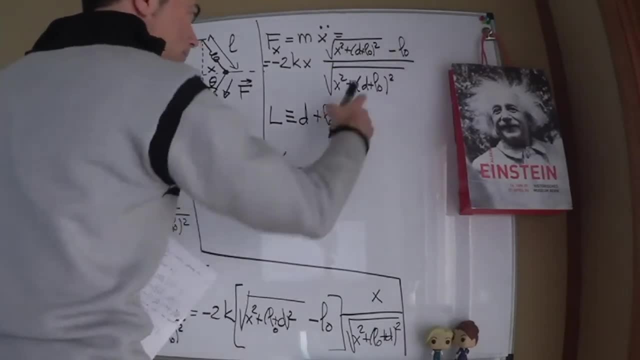 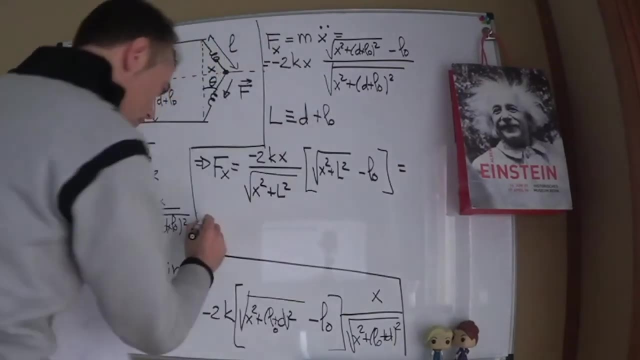 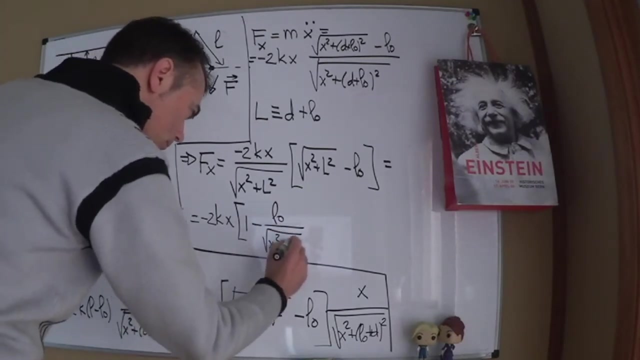 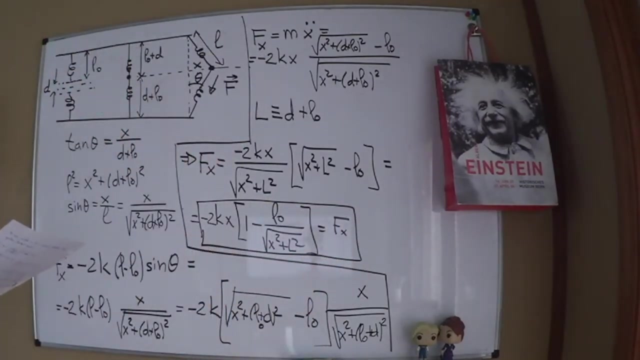 We take and rearrange a bit, dividing by this square root, So f sub x, is this minus two K x times this term here. So we have the mass of theta which is equal to minus two K x times this term here. 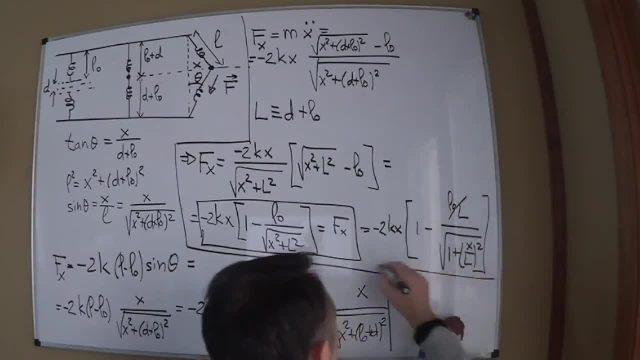 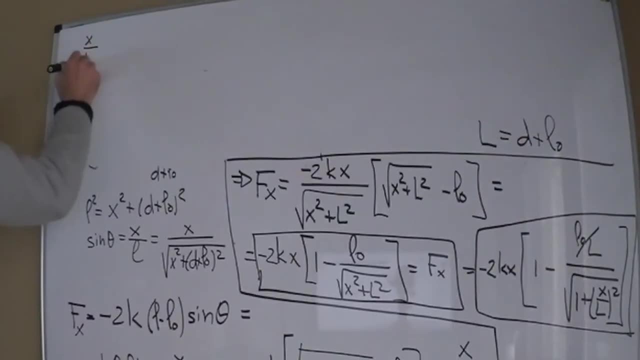 So f sub x is this minus two K x times this term here. So f sub x is this minus two K x times this term here. Now let's consider again small displacements. This means that x over capital L is much smaller. 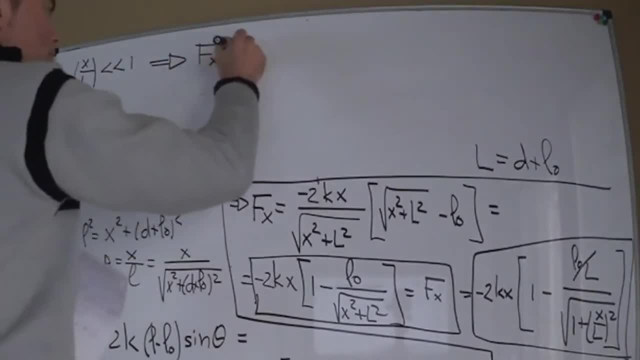 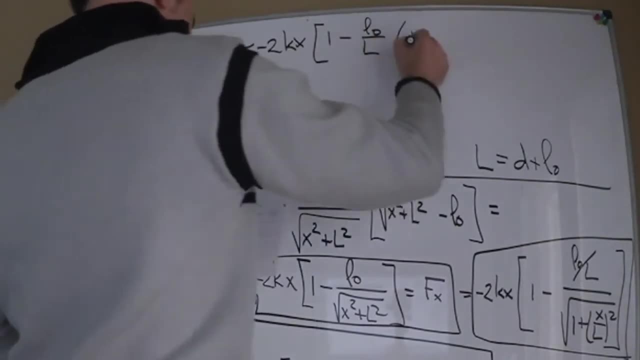 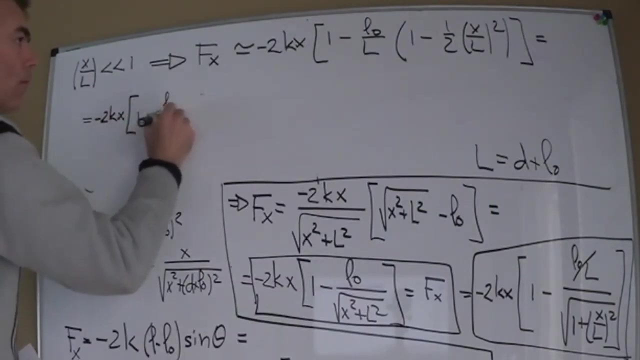 than one. so I can expand in series of Taylor that square root in that denominator For second order terms. For second order terms, Now I'll use that L0 is capital, L minus D, and do a bit of wibbly-wobbly-Matthews-tough. 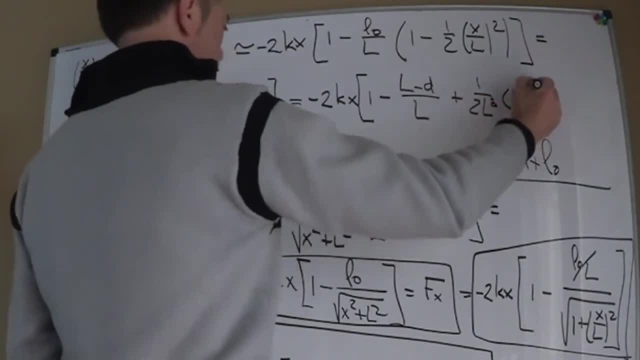 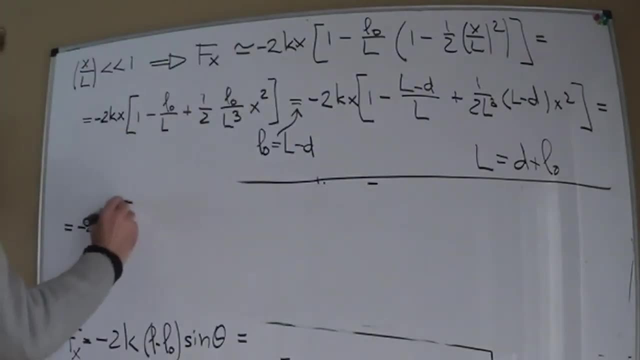 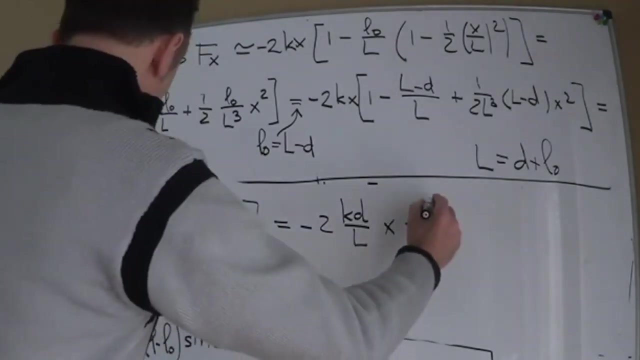 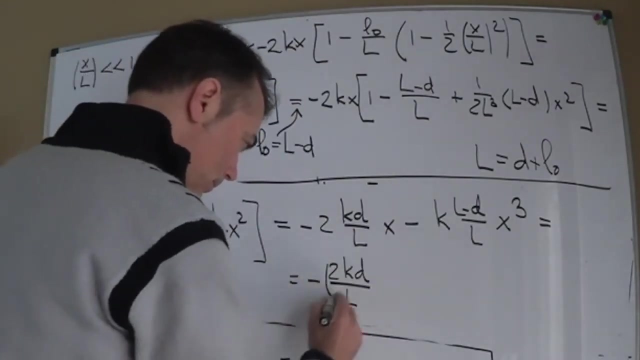 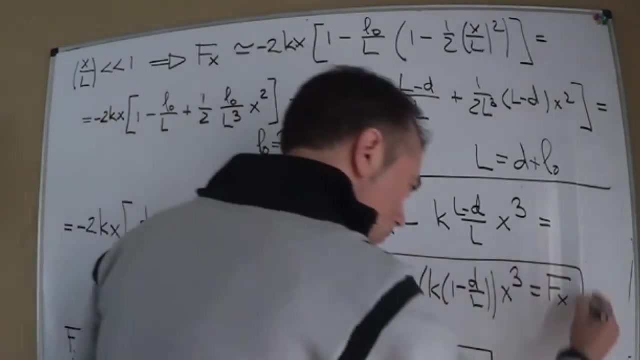 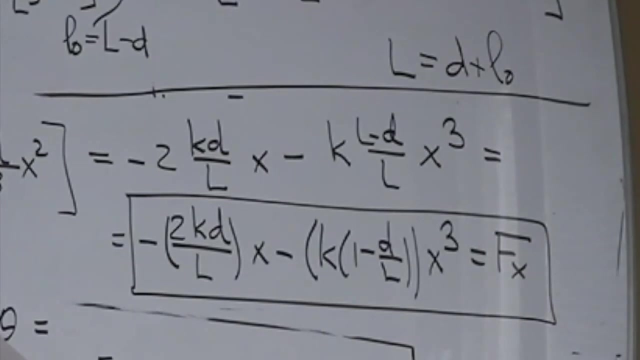 Wibbly-wobbly-Matthews-tough. So look at this. This is the force on the spring. in the limit of small initial displacement, We get the linear term, but this adds a term to the power of 3..